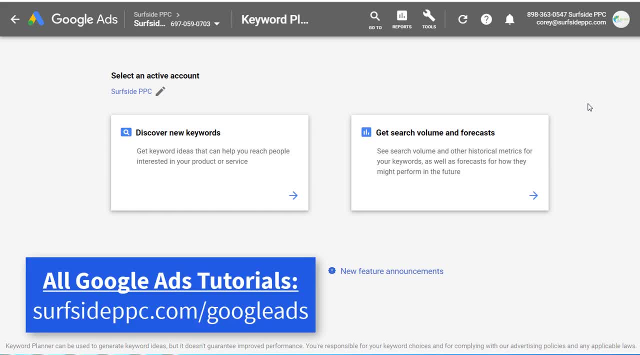 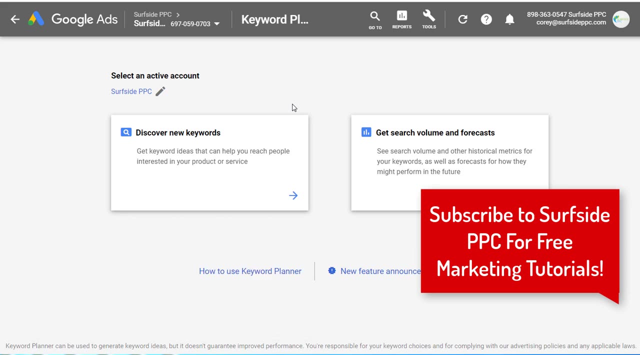 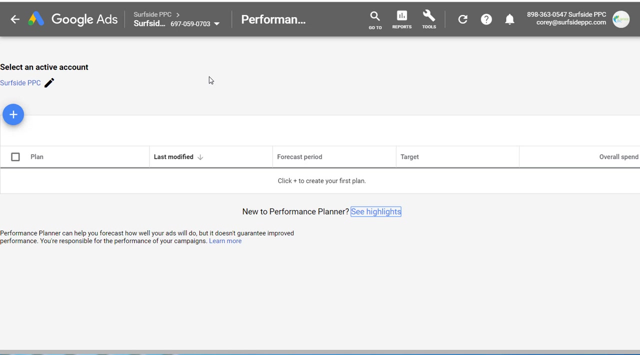 Alright, what's up everyone. Welcome to the Surfside PPC YouTube channel. Today I'm going to be going over Google Ads forecasting and budgeting and I'm also going to share a budgeting spreadsheet with you. So when it comes to forecasting, there's two different ways you can do it. You can do it using the keyword planner and building a plan in here. Otherwise, what you can do if you have an active campaign is you can use the performance planner. I'm going to create a completely separate video about the performance planner. It's a pretty new tool from Google Ads So you can see right here they have new to performance planner: see highlights. So, essentially, 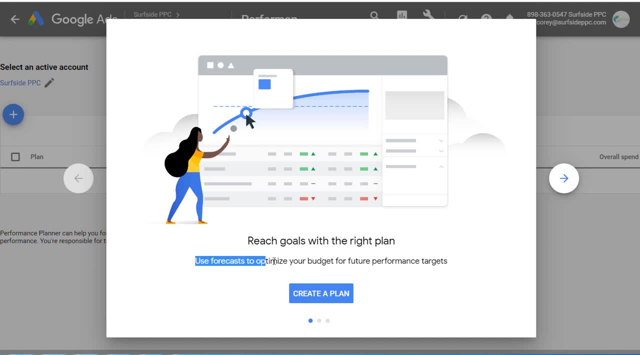 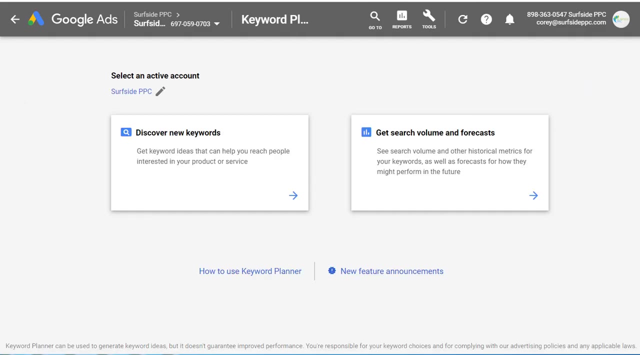 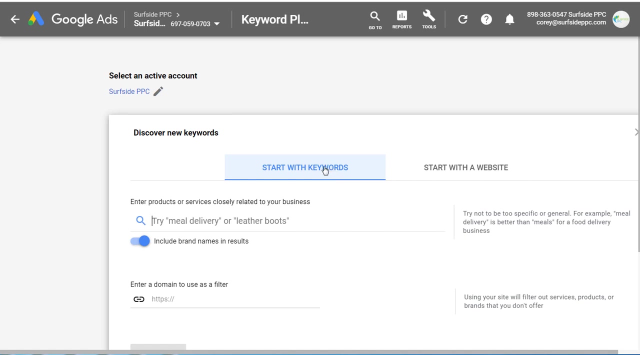 what you do is you create a plan and they're going to help you use forecasts to optimize your budget for future performance targets. So it helps you forecast your campaign and see how well a new campaign will perform, depending on the plan that you use. So I'm not going to be going over the performance planner here, So we're going to be coming back over to the keyword planner. So what I want to do is I want to click on discover new keywords And let's just say, for example, I want to create new campaign for my website, beachfrontdecorcom. I'm going to start with keywords here and we're just going to come in. I'm just going to 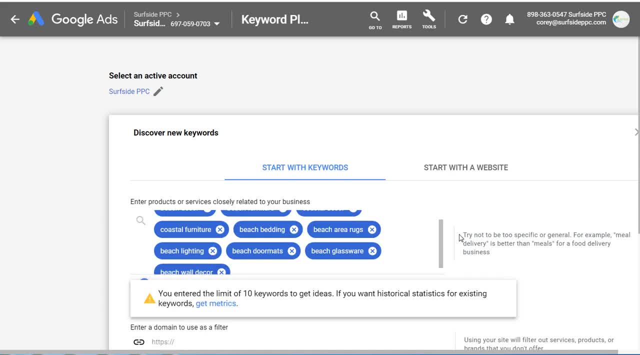 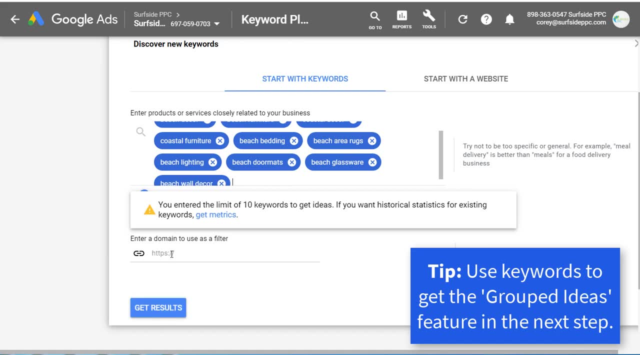 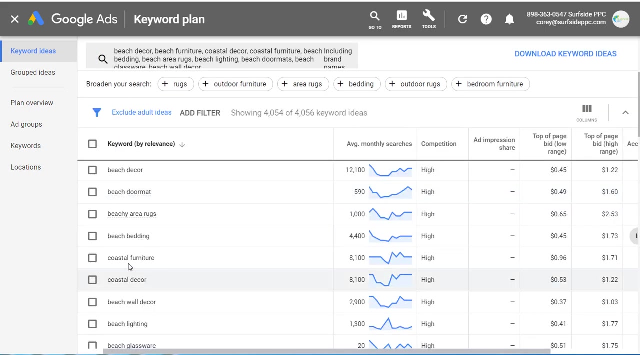 enter 10 keywords. Okay, so I entered 10 keywords here, So this is the most that you can enter at this time when you start with keywords, And what we're going to do is we're just going to scroll down and click on get results So you can enter a domain to use as a filter. if you want, You can start with a website as well, But with a website, you're not going to be able to use the grouped ideas that I use in the next step, So I'm going to click on get results now. Okay, so it's going to pull up the top keywords by relevance So you can see beach decor, beach doormat, beach area rugs, bedding. these are the ones that I entered. If I keep scrolling down, you're going to see there's more keywords down here. 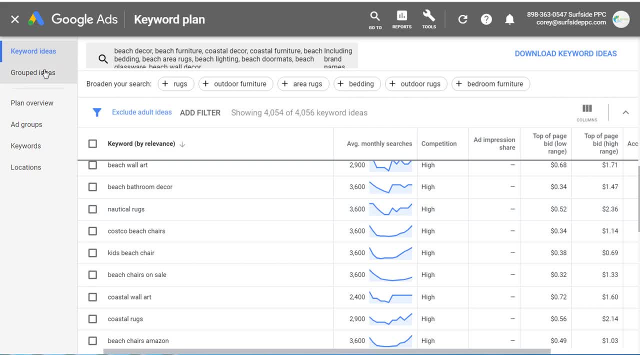 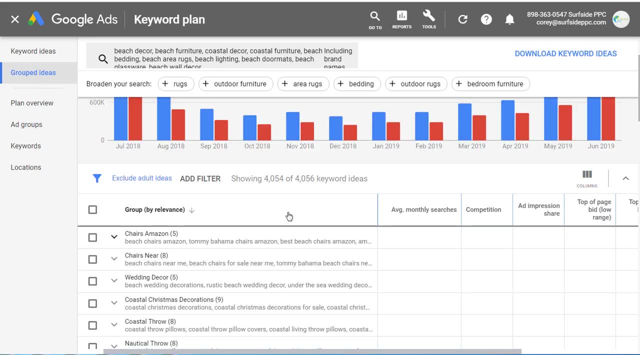 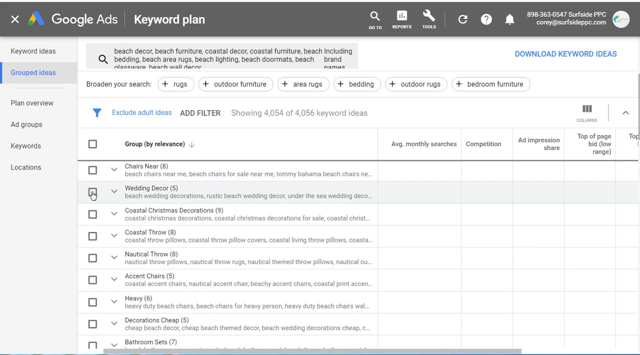 As well. So, basically, what we need to do is build a plan. So what I'm going to do is I'm going to come over here to grouped ideas. So in grouped ideas, what they're going to do is they're going to create a group by relevance. So these are ad group examples, So different things that you can use as you're building your campaign. So let's just say, I want to target wedding decor, So beach wedding decorations. I want to target all of these different keywords here. So we'll start there. You have coastal Christmas decoration. So let's say I want to target that as well. as we get closer and closer to Christmas, I want to make sure that I'm 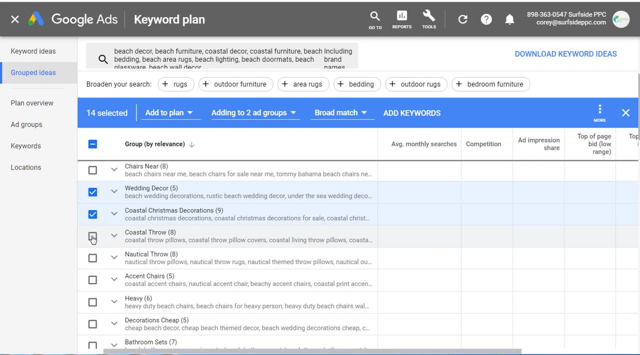 targeting these keywords- Coastal throw pillows- So we'll say I'll target that as well. So what you would do is you would add as many ad groups as possible that would be relevant for your campaign. As long as you have landing pages for these different ad groups, you should add them to a campaign So you can see right here I have add to plan. So it's going to say adding to three ad groups. So what that means it's in my plan. it's going to create three different ad groups for each of these grouped ideas below. Okay, so next is match type. They have broad match, phrase match and exact match. I generally use phrase match here because 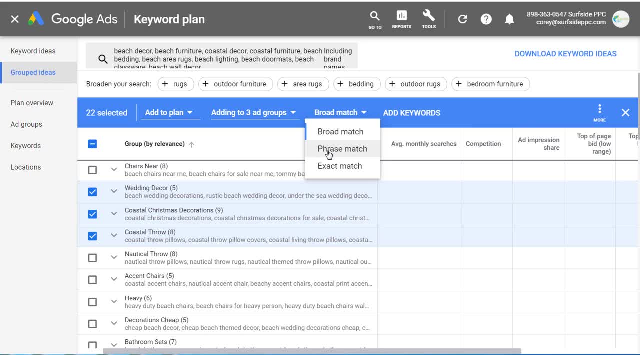 I think that's going to help match a lot of different keywords, match a lot of different search terms that people type in, but it's not going to be too broad, It's not going to be too exact. I think it gives me the most accurate forecast data. So I'm going to use phrase match for this, even though I don't really target phrase match keywords in my campaigns. I think it's the best to use for forecast data just based on the types of things that people are going to type in, because people aren't always going to type in these exact match keywords And I find broad match to just be too broad. So, rather than just adding these three ad groups right now, I'm going to create a few more ad groups. 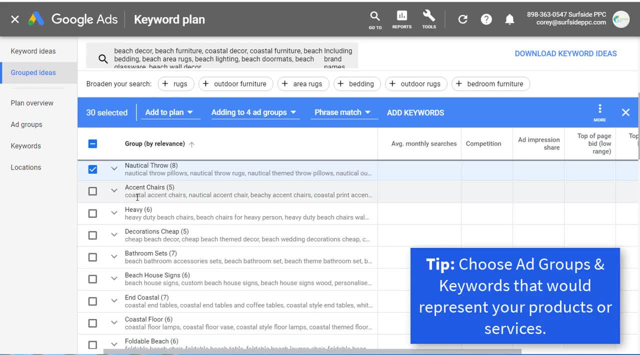 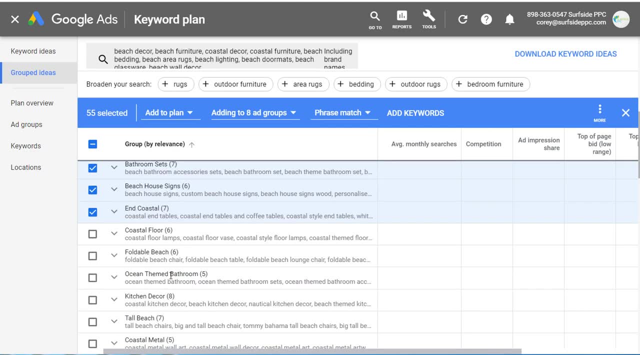 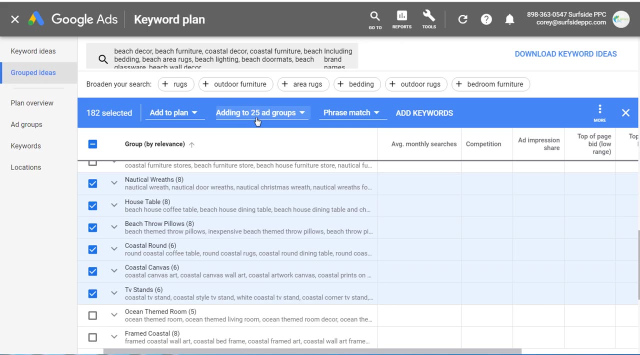 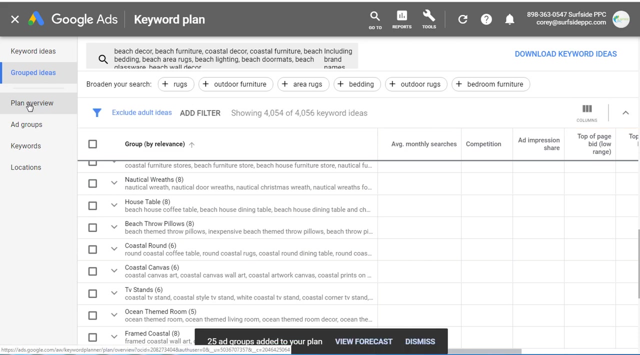 Here, just by clicking on these keywords, and we're going to keep scrolling down so you can see. accent chair- So we'll do that one as well. Beach bathroom accessory sets: We'll do that. Beach house signs. coastal end tables- Okay, so at this time we have 182 keywords selected. We're adding it to our plan. We're adding 25 total ad groups. Every keyword is going to be a phrase match keyword. So all we need to do is click add keywords and it's going to start building our plan here. Now you can keep building your plan if you want to go back into keyword ideas, If you want to make sure that your ad groups look good with all the keywords that you have. 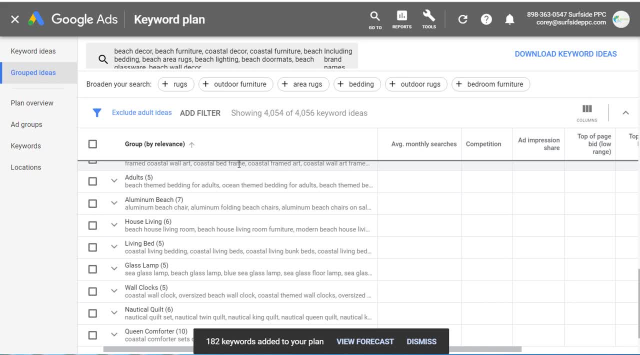 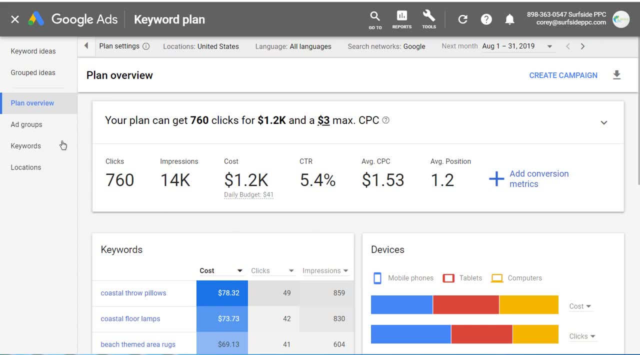 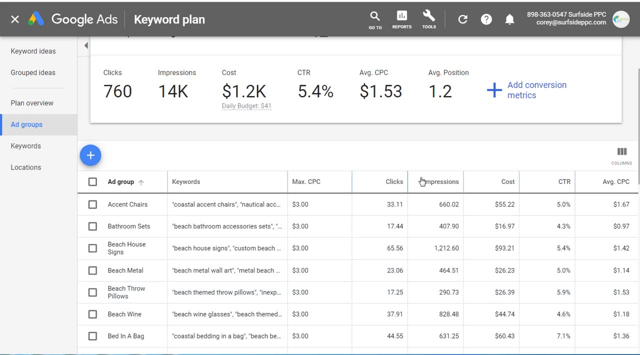 That are in there. I can add more grouped ideas here as well. So what I'm going to do is I'm just going to come over here to plan overview, and planning overview is going to allow you to forecast your data. So the other thing you can do is click on ad groups here. It's going to show all the different ad groups and show the max cost per click and how much they expect you to get from each individual ad group here. So usually things with more search volume. So let's just go by impression. So beach house signs, coastal throw pillows, beach themed area rugs- So they're basically saying these have more search volume than some of these other ones. 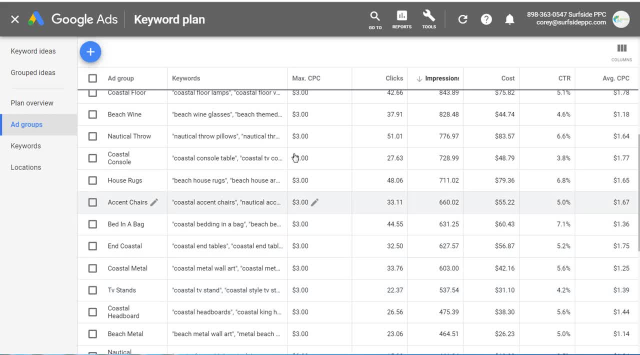 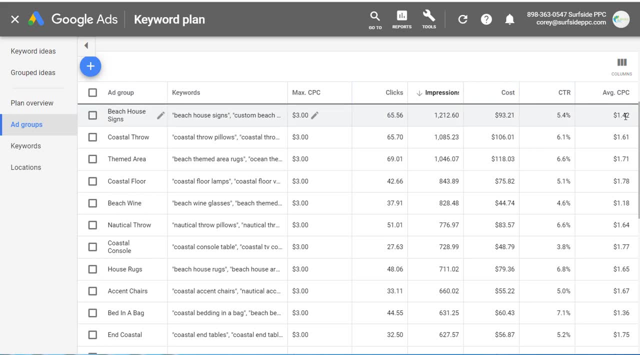 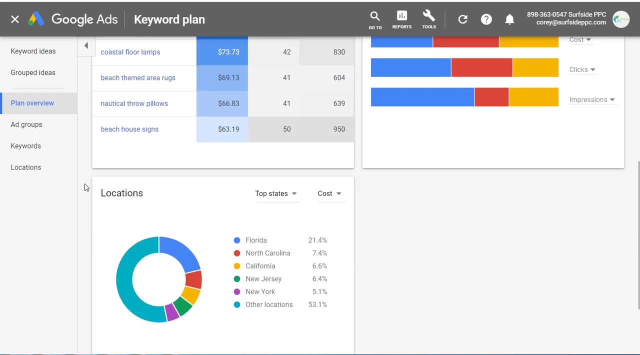 Down at the bottom and maybe they have a little bit less competition. because as you increase your max cost per click for a certain ad group, it's going to increase the impressions, clicks, the cost and the average cost per click for that ad group as well. So different ways to kind of look at the types of keywords that you're targeting by ad group. You can also do keywords and locations, But what I'm going to do is click on plan overview here and you're going to see it's going to show what they expect our top keywords to be, what they expect our top locations to be, by top states and by cost percentage. So we'll keep scrolling. 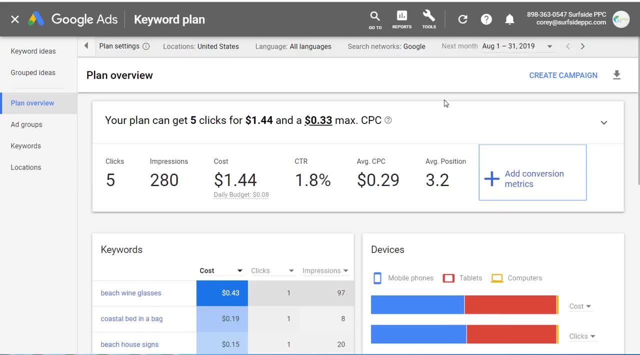 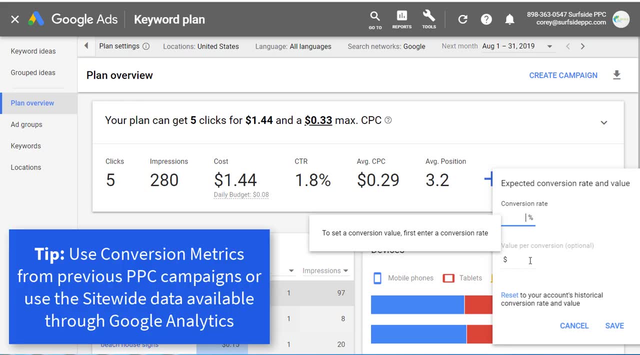 You can see devices here as well: Mobile phones, tablets, computers. OK, so one thing we can do is add conversion metrics here. So let's just say I use my site wide conversion rate and my site wide value per conversion. So let's just say my site wide conversion rate is four percent. So every 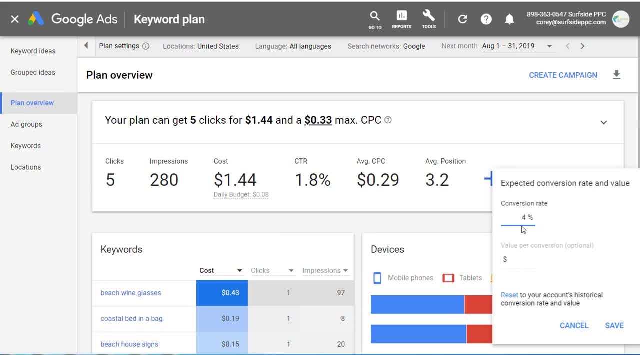 time, 100 people visit my website. four percent of people actually convert, and let's say my average value per conversion is seventy-five dollars, for example. Now we'll click on save. You can also reset to your account's historical conversion rate and value, so you can use that as well. 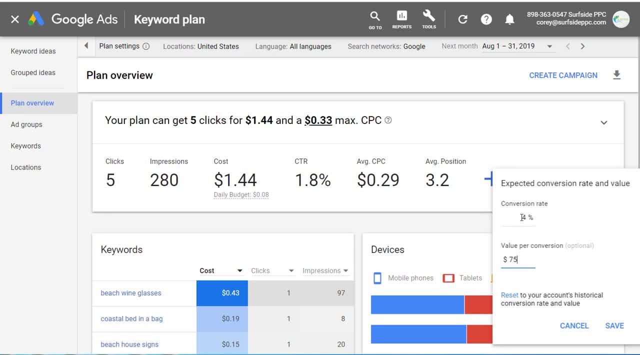 So what I'm going to do here is였 is just use this. you can get these, this data, from your google analytics account, so just go to the conversions tab, open it and look at your conversion rate, look at your value per conversion, and we'll click on save here. now we want to do is click on this drop down here, so i like to use this. 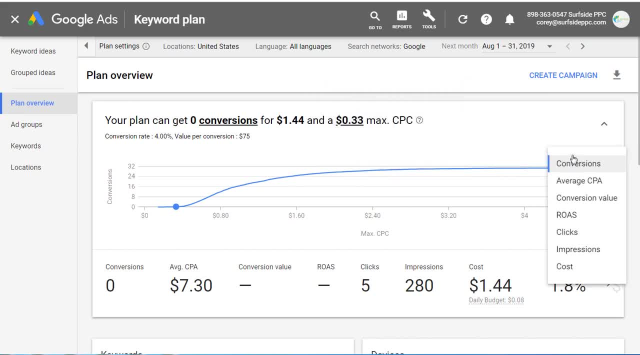 graph right here so you can see if you want to look at things like conversions, average cost per acquisition, conversion value, return on ad spend, clicks, impressions and cost. so let's just go to costs real quick and let's just say we're going to look at a max cost per click of here we go, 2.70. 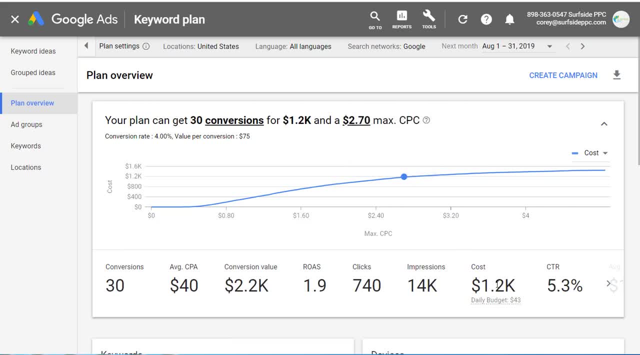 so essentially what that's saying is it will cost 1.2 thousand dollars for the month, so a daily budget of 43 dollars. it would give us 30 conversions, an average cost per acquisition of 40 dollars. so if our value per conversion is 75 dollars, then this would be a pretty good campaign. 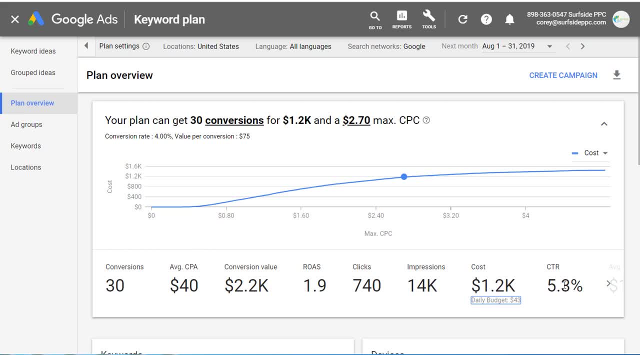 overall. so you can look at some different data here. it's going to say our click-through rate will be 5.3 percent: 740 clicks, impressions 14 000.. so the other thing you can do is look at return on ad spend. so let's just say, for example, we want to maximize return on ad spend. 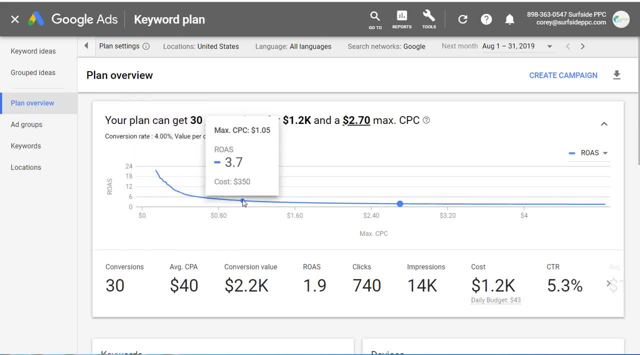 so you would kind of come over here and let's just say costs would be around 400- 420 here. our return on ad spend would be about 350 percent. so it's going to say our average cost per acquisition would be 22 dollars value per conversion, 75 dollars conversion value, about fifteen hundred. 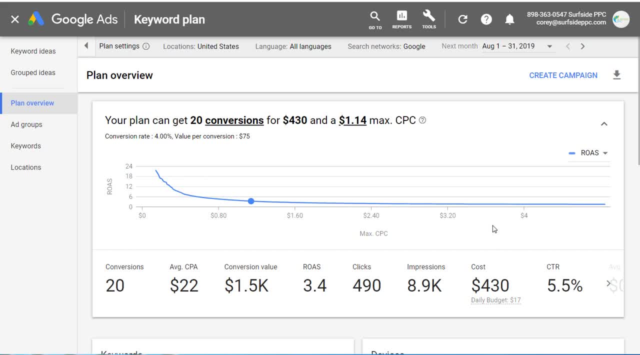 dollars with the spend of four hundred thirty dollars. so you can also just say: i want to get my return on ad spend, let's just say to 1.5. so it's not even going to show over here because we don't have enough volume. so let's just say our return on. 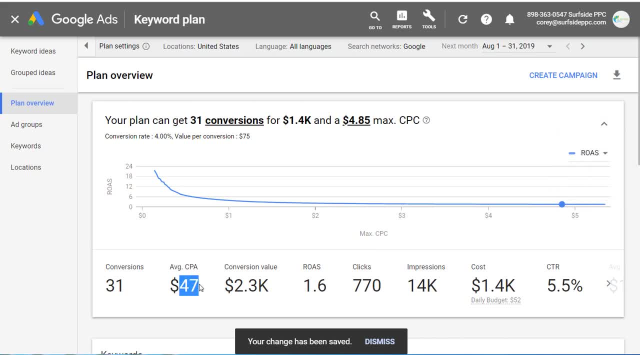 ad spend would be 160, average cost per acquisition: 47. we would spend about 1.5 thousand dollars daily. budget of 52 dollars. so it's a really great way to forecast your data using this tool here. basically, what you do is you build a plan using the google keyword planner you just come into. 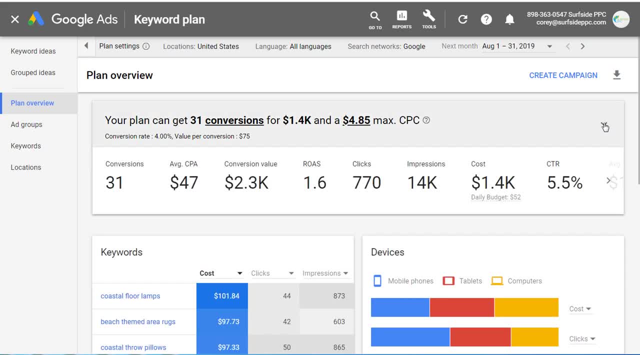 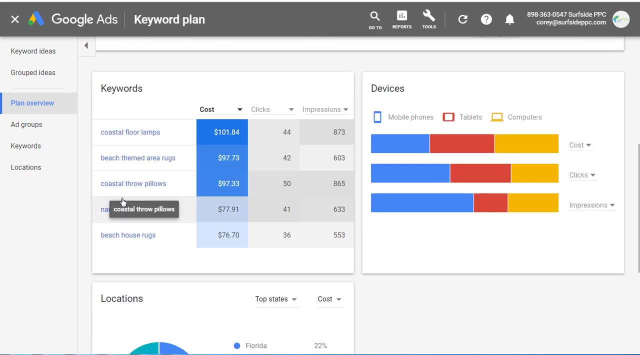 plan overview and then you're just going to click this little arrow and you can look at everything right here. by clicking on this arrow drop down, it's going to show your top keywords. so coastal beach, themed area rugs, throw pillows, nautical throw pillows, and again you have more location. 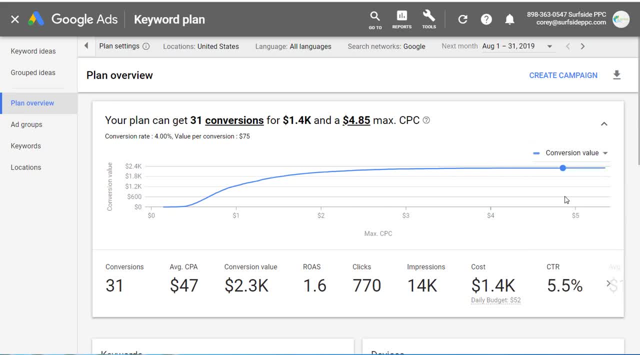 and device data down here as well. the last thing i want to go through here is conversion value. so in conversion value, which you can kind of see is your conversion value will go up and down and eventually reach a peak, depending on the types of keywords that you enter and, again, the more data. 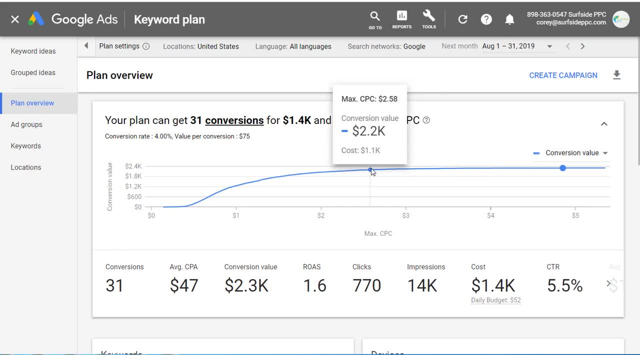 that you enter into your plan, the more keywords that you have, the more ad groups that you build, the better this forecast will be, and we can keep going down here a little bit. so it's going to show that maybe our best results will be somewhere in this line, right here. 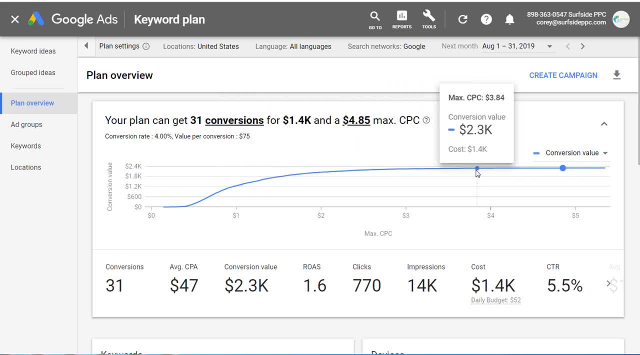 where we're not spending that much. we're not spending, you know, 1.5 thousand dollars, but maybe we come down here we're spending about seven hundred dollars. our conversion value would be one point nine thousand dollars, so it would be 25 total conversions we can drive for a total cost. of seven hundred thirty dollars, so this would be good results. i would probably build a campaign and i would look to start my budget somewhere between maybe five hundred dollars up to a thousand dollars, and then you can always increase it over time. you can keep adding keywords, so there's a. 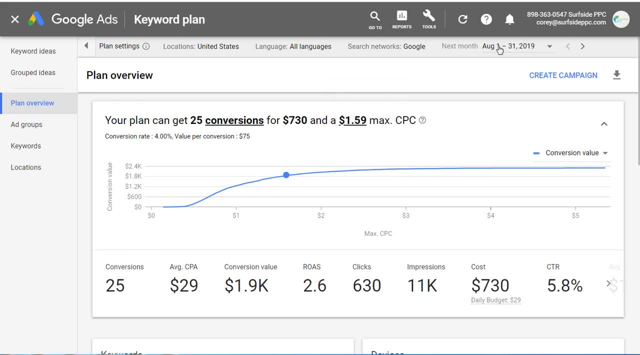 lot of different ways to do that, so this is how to forecast data. it's a really simple process. it's looking at a forecast for august 1st to 31st. search network is google language- all languages. you can update locations if you want. so if you're going to be targeting more than the united states, you. 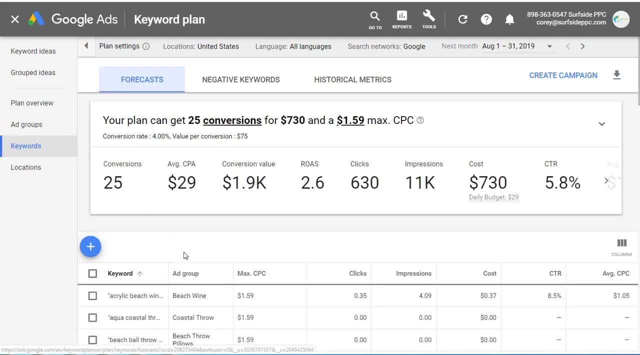 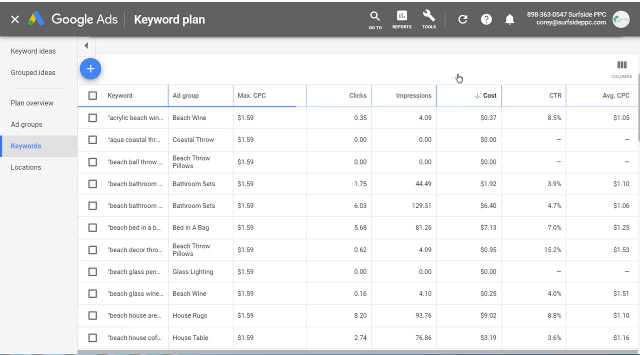 can do that as well. so this is a really great way. and then if we click on keywords- just one more time, i want to go through this real quick- it'll show some of the top keywords here, and if we go by clicks, impressions, so we'll just go by cost actually, so it's going to say our top keywords. 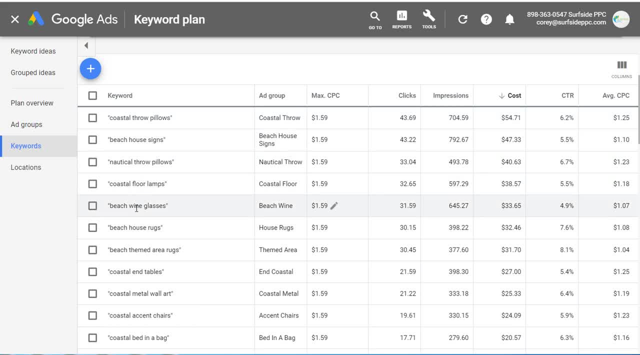 by cost will be coastal throw pillows, beach house signs, nautical throw pillows, and then we're going to go by beach wine glasses, beach house rugs. so a lot of different keywords here, and it will give you an idea of what you're going to be spending your budget on. so the more keywords that you add here, 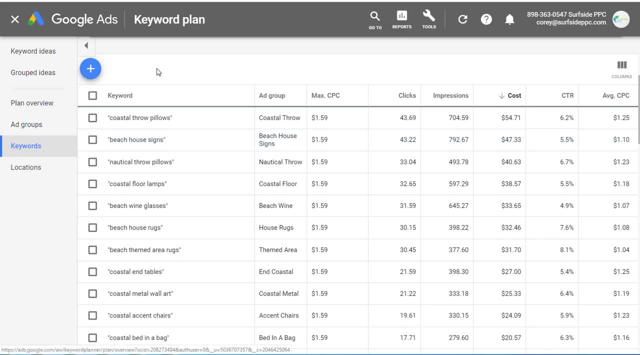 the more ad groups that you create in your plan, the better your forecast data will be. so now, last but not least, i want to go through budgeting and i want to share with you a free budgeting google sheet that i'm going to put in the video description for this url. also, leave it as the 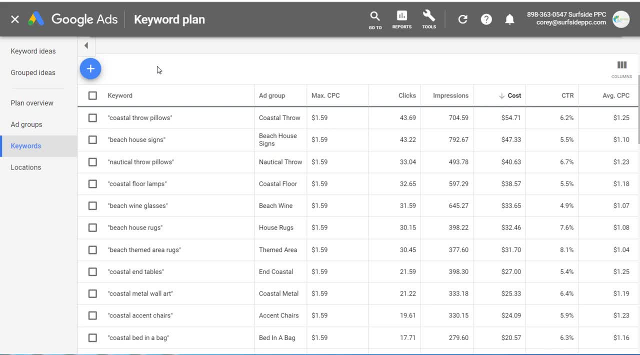 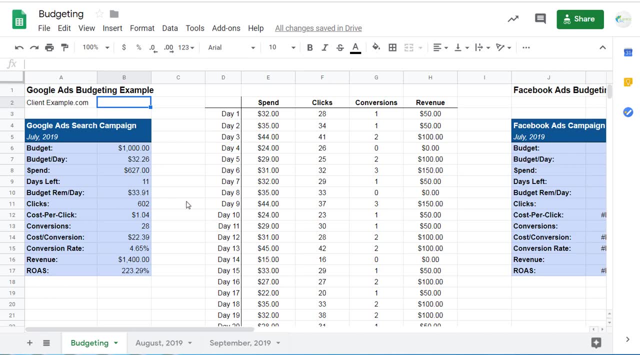 top comment on this video so you can easily find it, download it and use it yourself. so, with budgeting, so as you're running a campaign, this is the type of budgeting spreadsheet that i use and i update it daily. so what i'll do is you can see, i have my google ads search campaign. it's a google ads. 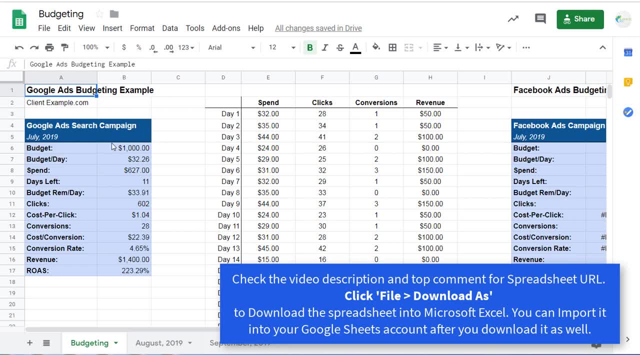 budgeting example for clientexamplecom down here. so this is the main thing. it's going to say budget. so total budget for the month, budget per day. so you're going to take the budget divided by the amount of days in that month. so for july, total spend so far. so this is. i'll show you this in a 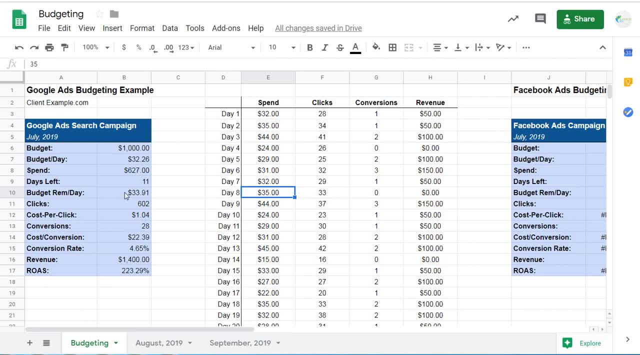 minute days left, so 11 days left in the month budget. remaining per day: 33% per day, 33% per day dollars and 91 cents. so clicks- this is going to be total results, clicks, cost per click, conversions, cost per conversion, conversion rate, revenue and return on ad spend. so you kind of keep track of. 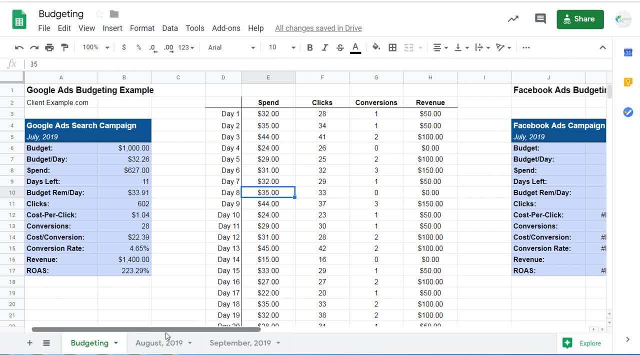 everything that's going on in your accounts, and you can do the same thing for bing ads. you can do the same thing for facebook ads. if you're running a google ads search campaign and a google ads display campaign, maybe a google ad shopping campaign, you can look at all of those as well. 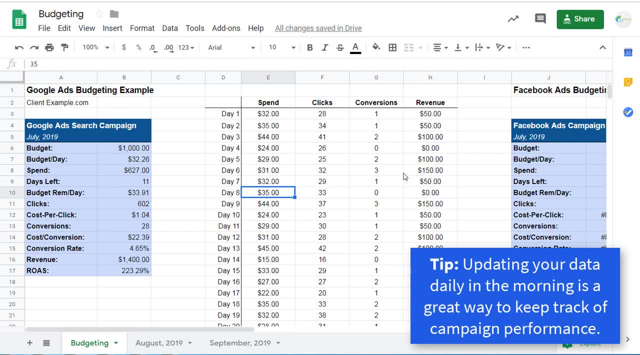 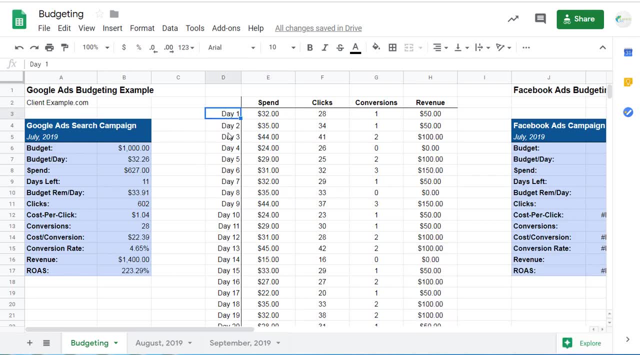 and look at spend, clicks, conversions, revenue, see how the campaign is performing over the course of the month, see how your budget is going to be over the course of the month, see how your budget is pacing. so now, what i'll do is i'll look at each individual day, so i have day one, day two, day three. 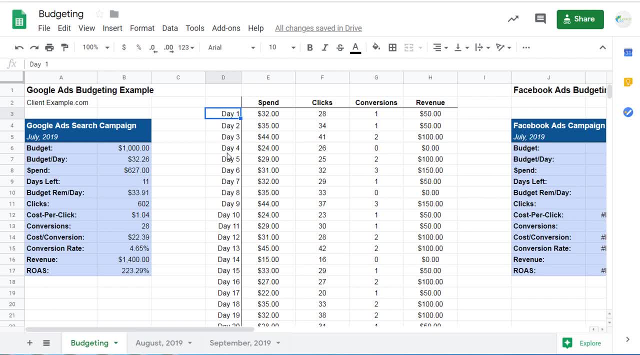 generally, you can put the actual dates here, so july 1st, july 2nd, july 3rd, july 4th, and then what i'll do is i'll take the previous day's worth of data and put it right in here. so today is july. 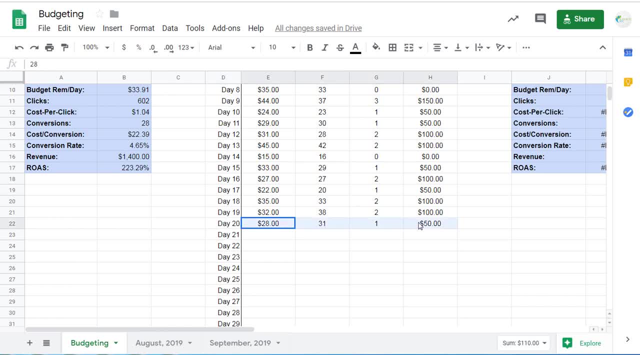 21st, so i actually need to do july 20th. so i'm going to take this data right here. we're just going to get rid of it for right now, and then what i would do is i would open up my campaign, so you 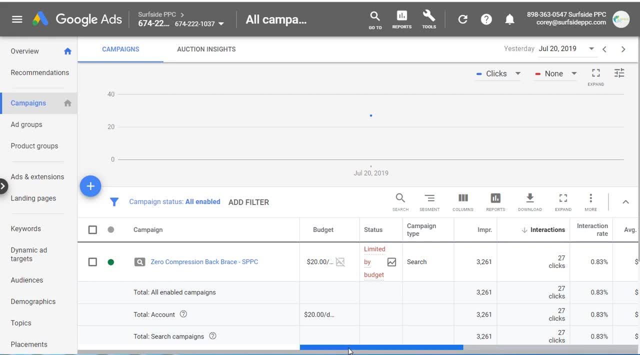 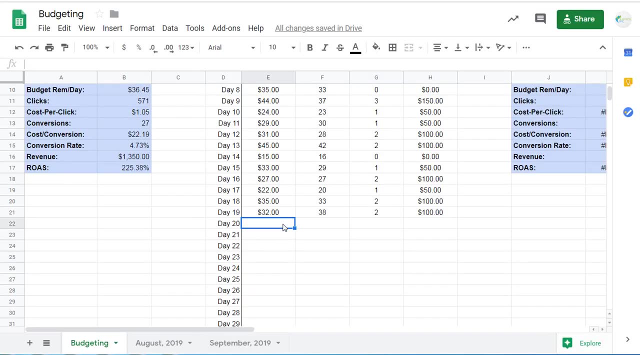 can see i have my campaign open here. so i'm just looking at a search campaign and let's just say, for i have 27 clicks from yesterday, 1886, so i'll just come over here. so i spent 18.86- drove 27 clicks. 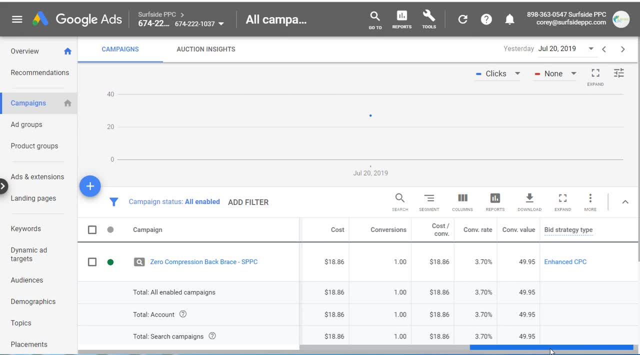 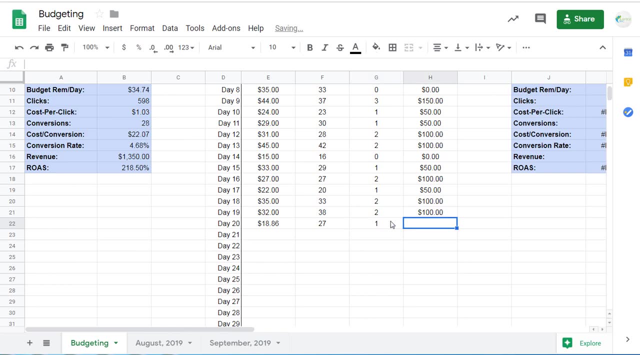 and then we'll come back over. keep looking. so we drove one conversion and the conversion value was 49.95, so we're going to come over here again to budgeting. one conversion conversion value was 49.95. click on enter. so now we'll update this over to the left hand side, so you. 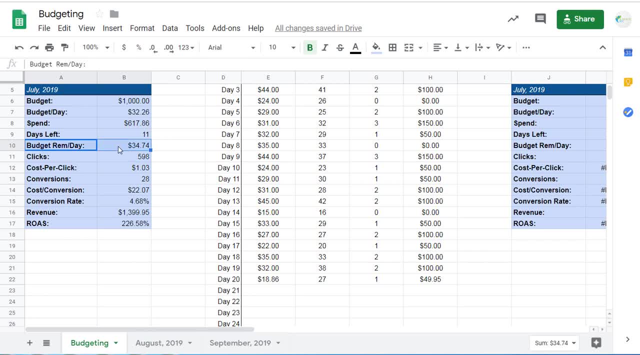 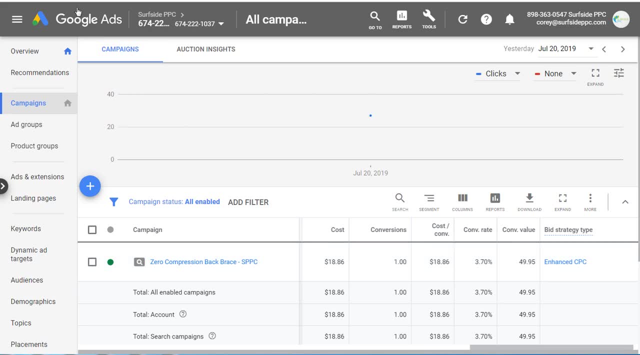 can see, our data might have changed a little bit, but it's showing my budget remaining per 34, so you would want to make sure that your campaign is pacing correctly for the month. now, really, what i would do is, if i know that i have a 1 000 monthly budget, then i'd probably set 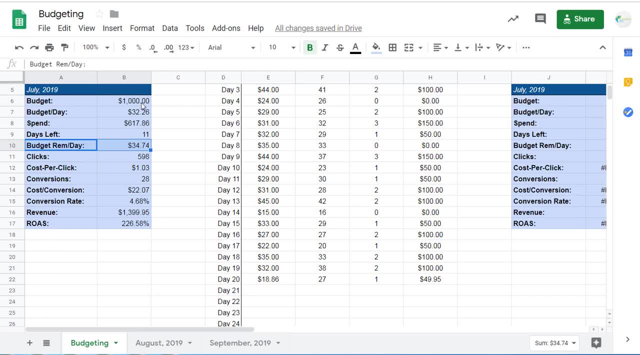 my budget at around 33 dollars per day, because then i'd spend around 999 for the month. so that's really how i would do it: make sure you're spending it and pacing it correctly. this is just sample data. it's not data from the actual campaign, but it's a great way to look at your performance over. 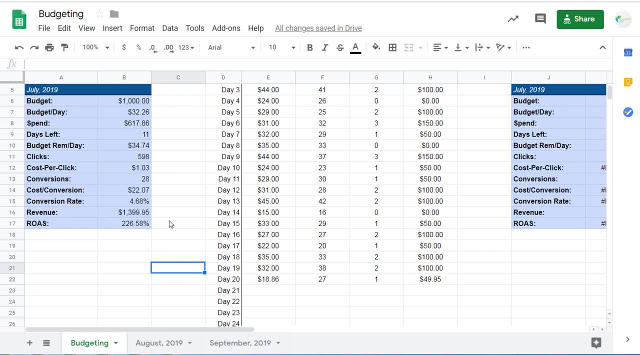 the course of the month and then just by updating each day. so if you're running a google ads campaign, if you're running multiple campaigns for the same client and you have multiple clients that you're managing, it's a great way to look at how things are pacing, how the previous day went. 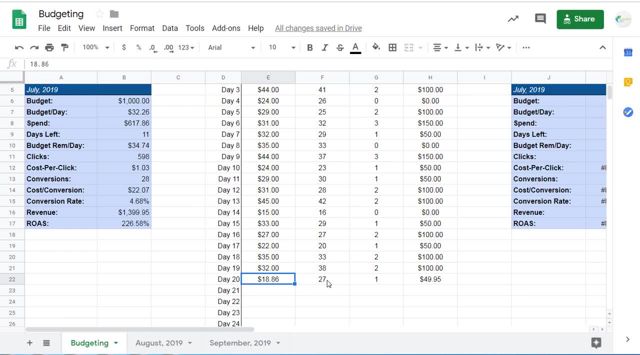 i usually start my morning doing this. so you wake up, you enter the spend for each client, the clicks, the conversions, the overall conversion value that drove, so you don't need to worry about it too much on a daily basis, but as you start doing it on a weekly basis, so you look at day one to day seven. 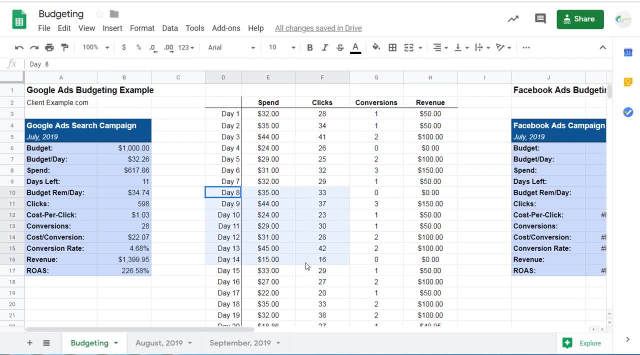 see how the campaign is pacing for the month. look at day 8 to day 14.. so you can kind of look at all. i like to just update it every single day and then you're able to see how your budget is pacing, how many clicks you're driving, how many conversions you're driving, what your return on ad spend is.